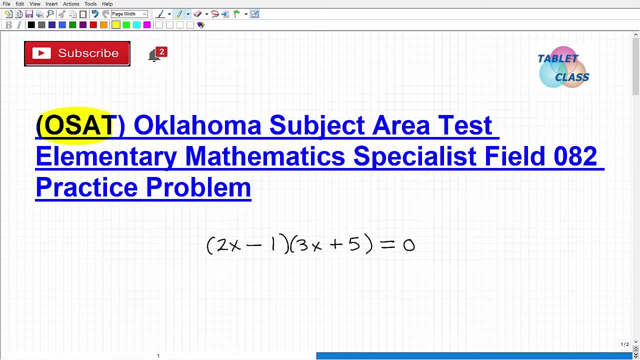 Okay, let's talk about the OSAT or the Oklahoma Subject Area Test, but we're looking at one specific test in this video and it is the Elementary Mathematics Specialist exam, and that is field 082.. So it's very specific and teaching, no matter what state you're. 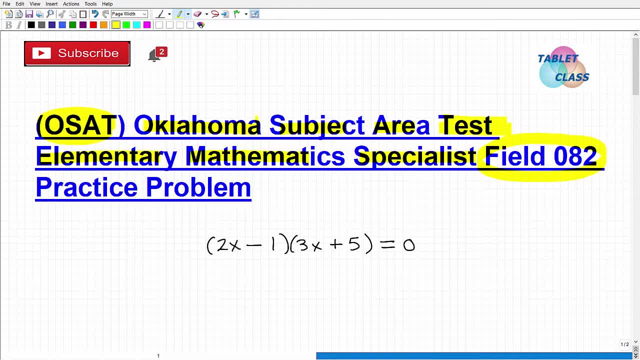 in. there's very specific teacher certification exams. So there's not just one for elementary, there's not just one for middle school or high school. Sometimes there kind of is, but you really need to know what specific test you need to teach. you know at the school. 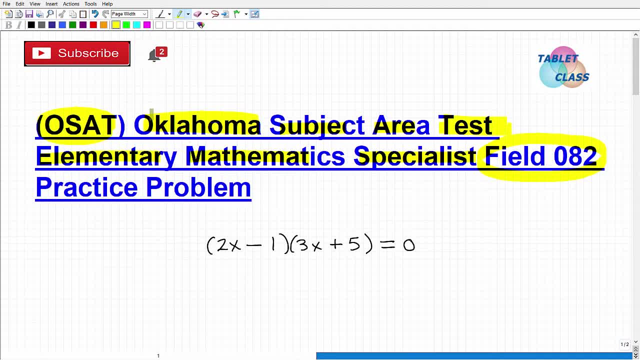 or job that you want to get into. So we're looking at this particular test and we're going to do a practice problem on the level of math that you should know to handle this particular OSAT test. So let me go ahead and just first introduce myself. My name is John. 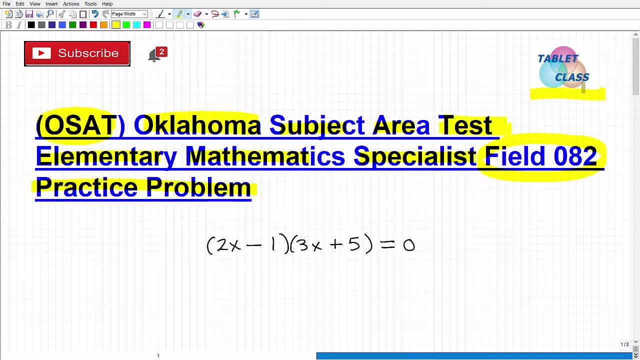 I'm the founder of Tabic. I'm a class math. I am a middle and high school math teacher, so I definitely know what it's like to teach, teach in a classroom and take certification exams. So, as a middle and high 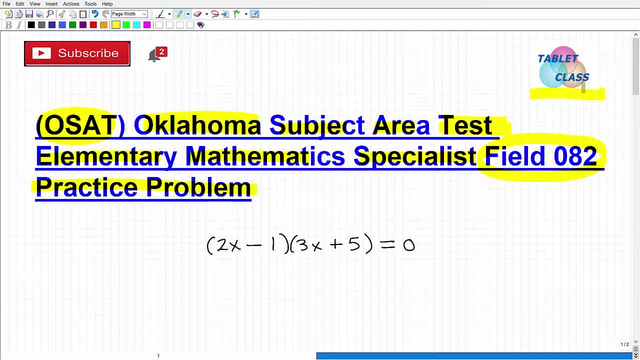 school math teacher. the exams that I've had to take, those are pretty challenging and I even have a degree in mathematics and a master's degree, and even then you still need to study. So you have to study for these exams, and here especially with the elementary. 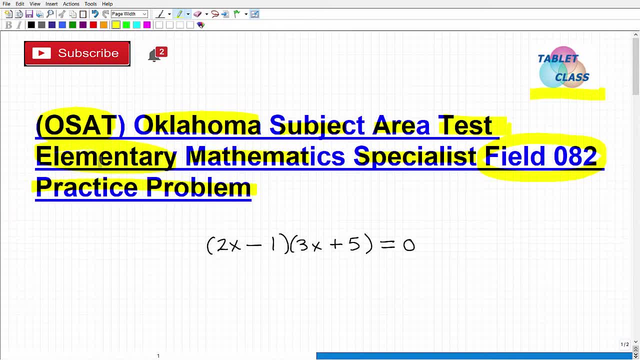 level test. I think some people can get thrown off- and I've heard this before with a lot of elementary teachers and it's no fault of their own- When you hear the word elementary and you say, well, I'm only going to be teaching. 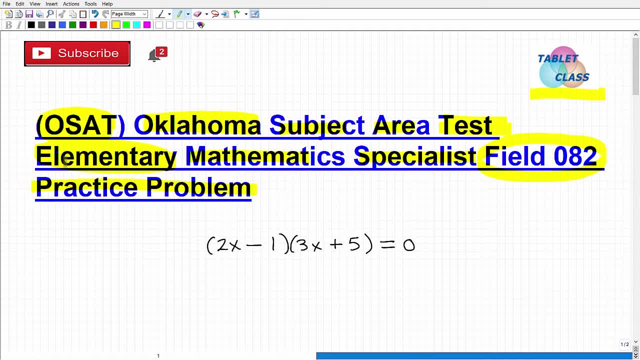 elementary level math, or you know, I'm at that level of K through five. whatever the case might be, you think, well, I'm not going to have to deal with algebra, geometry, you know more advanced math. but that's not the case, at least on these certification exams. 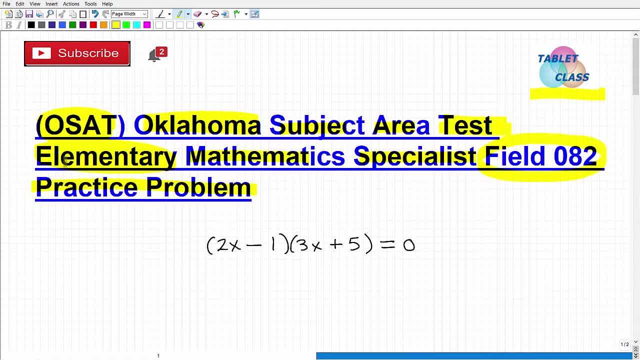 Many exams- this one in particular- you're going to have to know what I would classify as high school level math. You're going to have to be really strong in algebra, geometry concepts, and not just at a general level either. You're going to have to really brush up on your math skills and if you were weak in 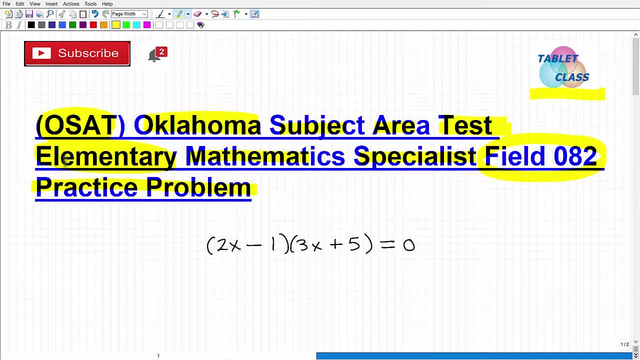 high school math or in college, math, then you're going to want to put some extra effort in to get ready for this test because you don't want to go in and take your exam and fail. okay, Many teachers have to take certification exams multiple times. 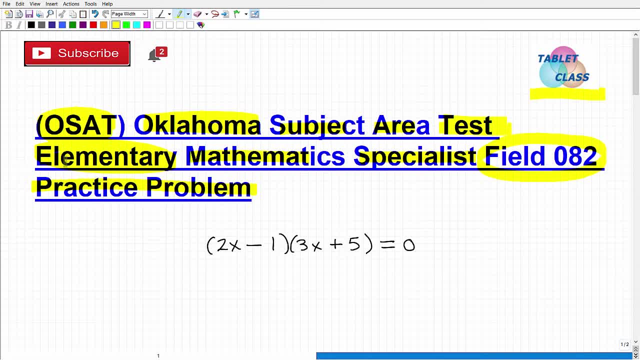 That's kind of common or normal. I think. not every single teaching candidate or teacher passes every exam the first time out, so you just don't want to, you know, be in that situation if you can avoid it. But that being said, I want to let you know that I have an excellent math prep course. 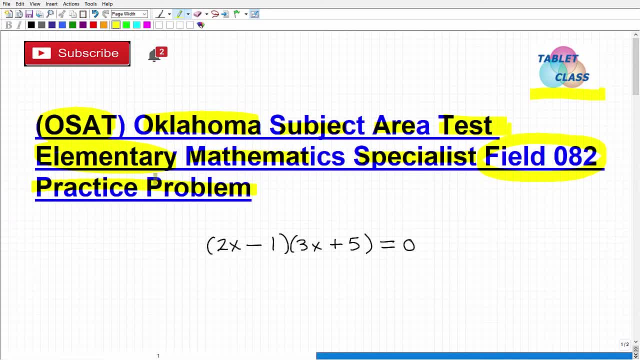 for the OSAT elementary math, specialist field 082.. I'll leave the link to that in the description, but we'll talk about that later. What I want to do is take a look at this nice little practice problem, and this is something. 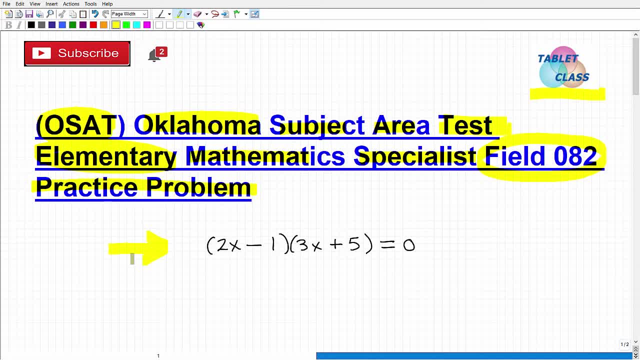 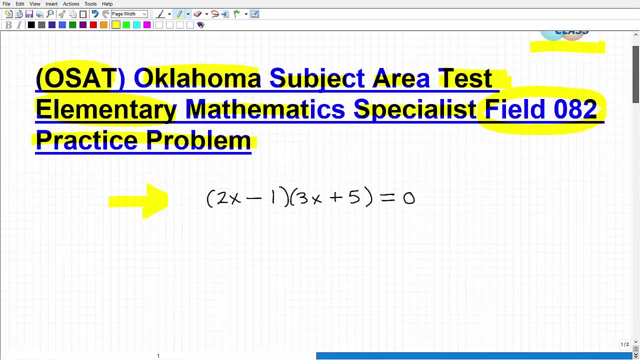 you should definitely be able to handle That, or be comfortable with, at the level of math you're going to have to know for this particular OSAT exam. All right, so what are we talking about here? Well, this is the problem. 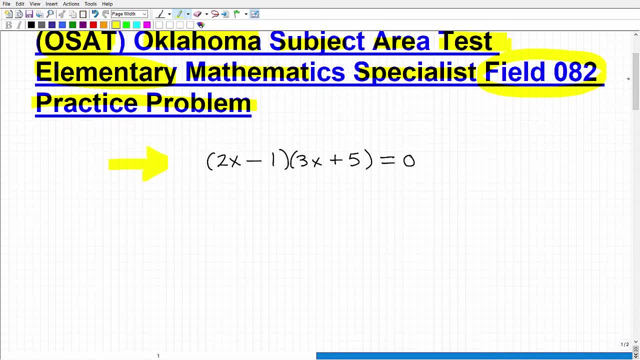 Of course I'm going to solve it, and it's an algebra problem. I'm not going to give you too many hints because I want you to take a crack at it. So even if you're not sure what to do, okay, you should still think about it, okay. 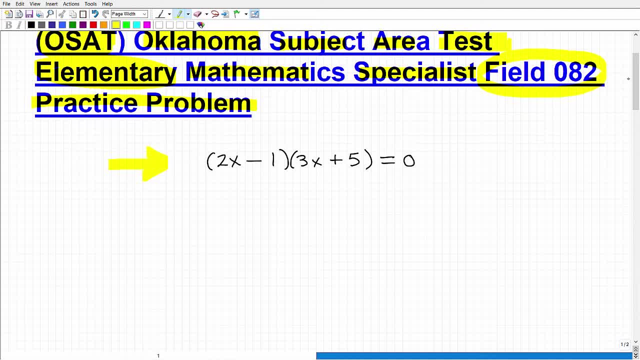 Just think about it for a moment, or go ahead and pause the video and actually solve it, or tinker around, Whatever the case might be, because I'm actually going to explain it here in a second. Okay, so let's get to the solution here. 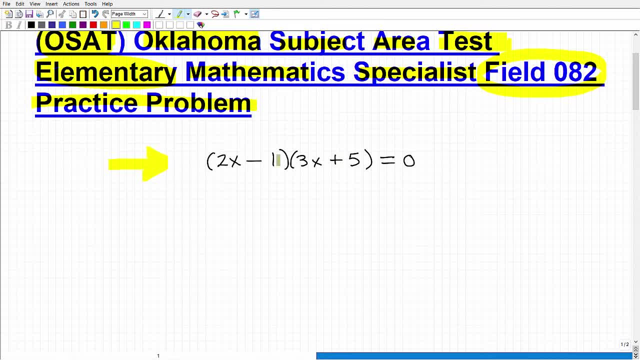 So what we have this is actually a quadratic equation that's been factored okay. Now, if you remember, the quadratic equations are things that look like something like this: 3x squared minus 10x plus 7 equals 0, something along this format. 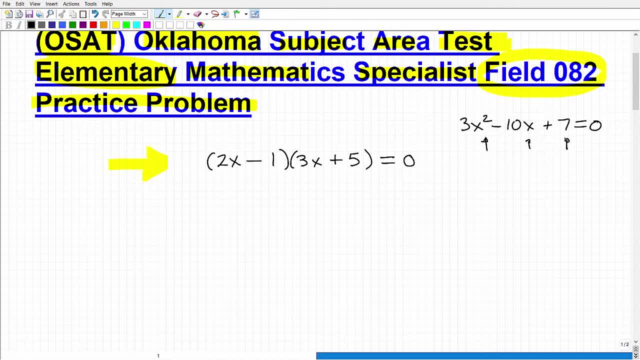 And you have this x, You have an x squared, you have an x and you have a number. And if you think back to your math days, whether that be in college or in high school, for sure, and you wouldn't be taking this exam if you didn't take the math that you already need- 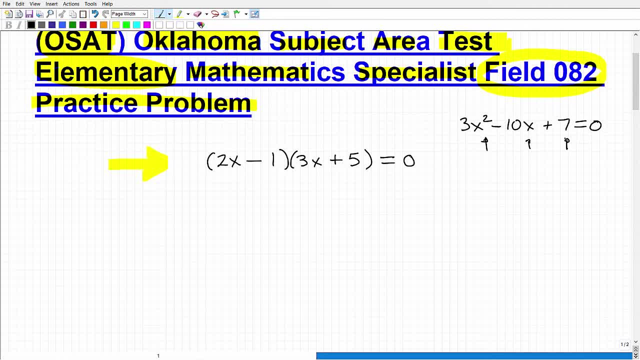 for this particular OSAT exam. In other words, you're going to be a teacher. You've definitely taken algebra, geometry et cetera. So if you recall to solve a type of equation like this, there's various approaches that. 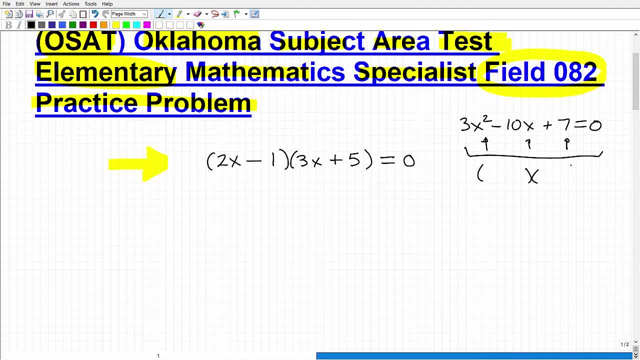 we want to do. One of the first things we want to do is see if we can factor, Good, okay, And if we can't factor it, we move on to the quadratic formula. and then there's other techniques as well. So in algebra, solving equations is a huge skill you need to know. 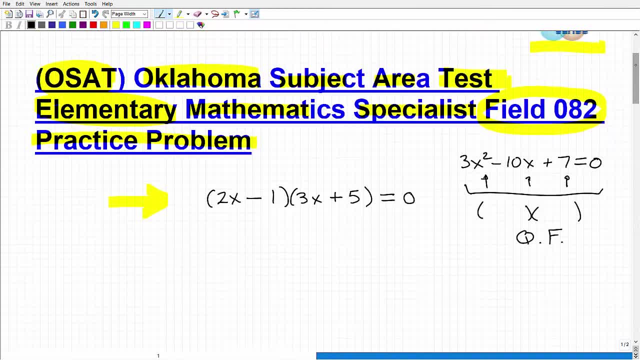 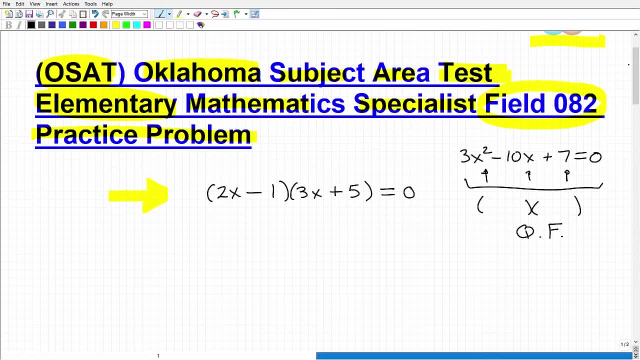 And I would say, for this test, you're going to have to be able to solve various types of equations, quadratic equations being one of those type of equations that you're going to have to solve. Okay, so here, for example, if I have this quadratic equation, 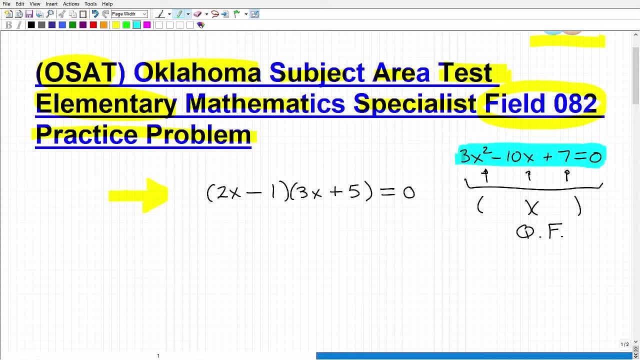 And it's set equal to zero. Again, I don't want to turn this into a full lesson, because this you know one. it wouldn't. I wouldn't have enough time to really teach this to you quickly, But just kind of, you know, trying to brush off any cobwebs in your memories. 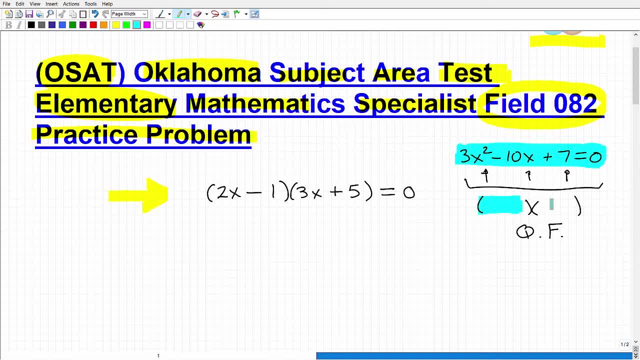 But anyways, if this is set equal to zero, I can factor this, hopefully, And that's always the easiest thing to do. Of course, that's assuming you know how to factor polynomials, All right, so let's get back to our situation here. 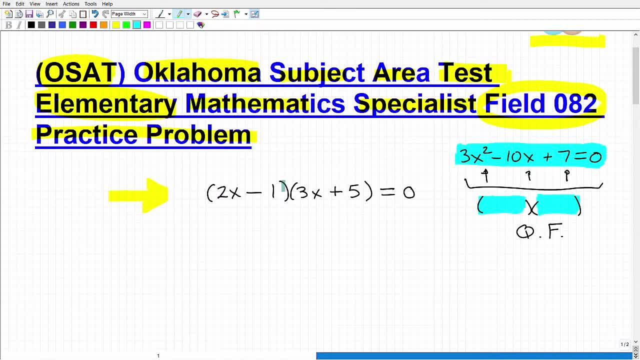 And I kind of gave again. it gave you a problem. It's nice and easy. So I have one factor here, one binomial, we call this, And it's being multiplied by another binomial. Now, if I multiply these together, I would end up with something like this over here: 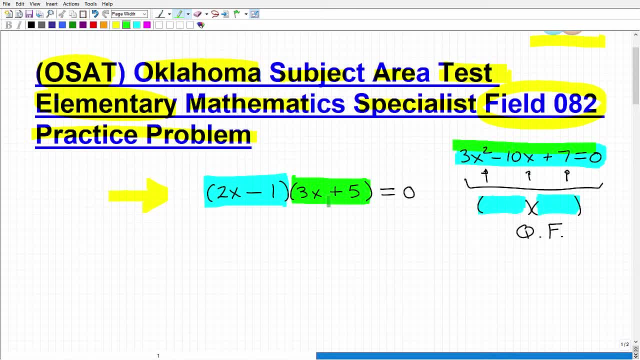 Okay, now we're not going to do that for this particular problem because that's not necessary, right? So this is your problem. on your test, You don't need to look at the original problem, You just need to look at the factors. 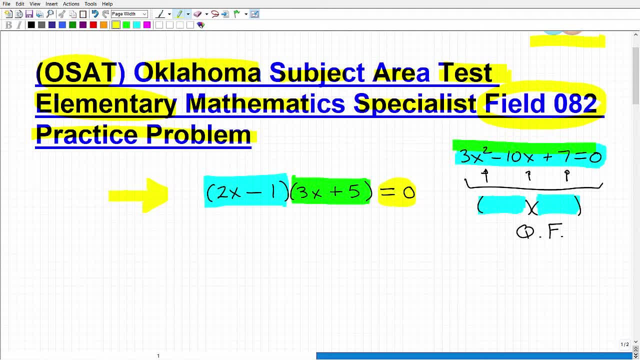 And the most important part of this problem is, you see, that This is equal to zero. All right, so what we have here is one thing, something okay, this quantity being multiplied by this quantity. In other words, let's think of it this way: 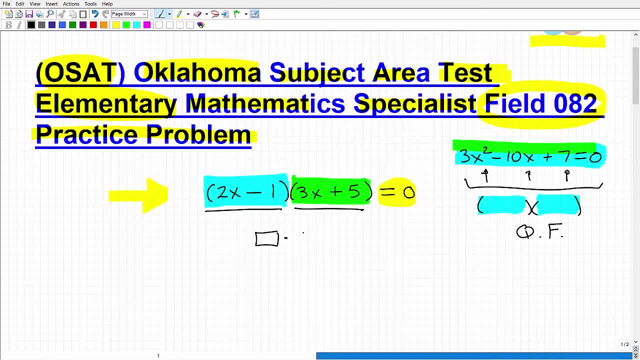 I have something- let's just call that a box times- something else- Let's call that a triangle- And that's equal to zero. So what I want you to do is just let's think of this question here for a second. I have something being multiplied by something else, and that's equal to zero. 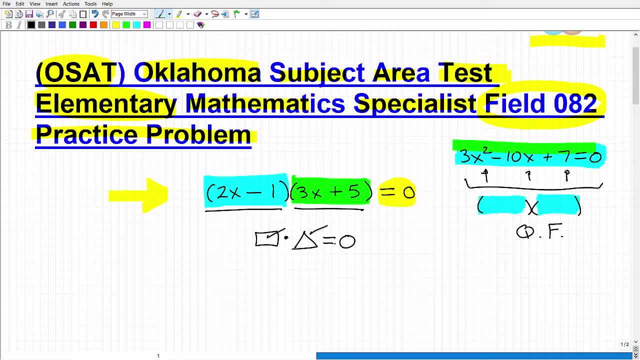 Now think of it this. Let's say I'm seeing you on the street and I say, hey, listen, I have these two numbers and when I multiply them together, my answer is zero. all right, So I would say, hey, can you tell me what these numbers are? 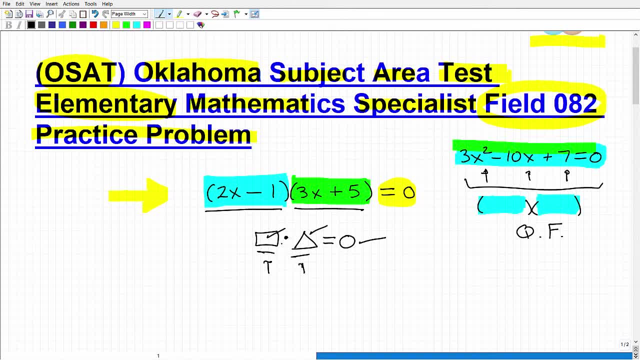 And you would say: okay, the only way you're going to get zero. if you're multiplying two numbers together and you get an answer: zero, one of these things has to be zero, right? One or both have to be zero. That's the only way you're going to get a product of zero, okay. 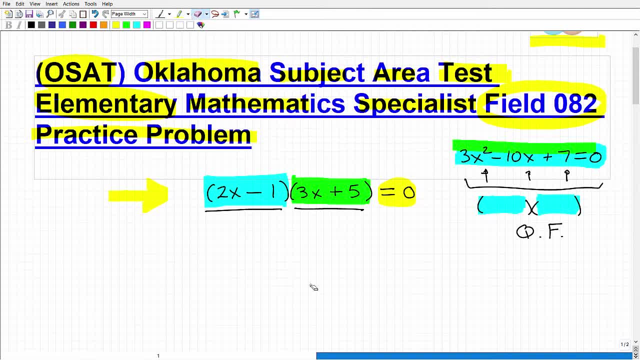 This is something called The zero product property, which is a wonderful property in math because it makes our lives so much easier. So that's why we want to be able to factor And when we have this thing set equal to zero, I can say, okay, this thing times, this thing is equal to zero. 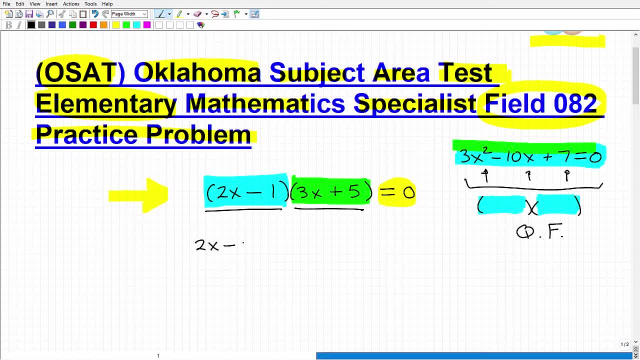 I can set each factor equal to zero, right? So 2x minus 1 is either got to be zero, or 3x plus 5 is either got to be zero or both are zero. Now, one thing about Quadratic functions or quadratic equations is that there will always have two solutions. two solutions: 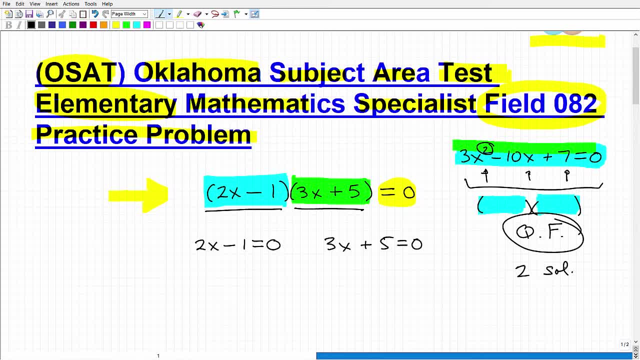 Now those solutions can be what we call real numbers and or complex or imaginary numbers. Now this is getting kind of a little bit more advanced. okay, I could spend a lot of time talking about this, but you're always going to have two solutions when you're dealing with quadratic equations. all right, 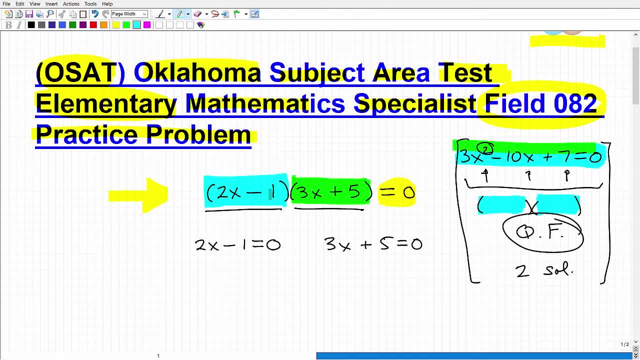 Not just one. All right, So here, now that we know this, all I have to do is solve these respective equations here. nice and easy equations. So if you couldn't set up the problem, if you didn't know what to do here in this case, why don't you go ahead and pause the video and see if you can solve these two little basic equations here? 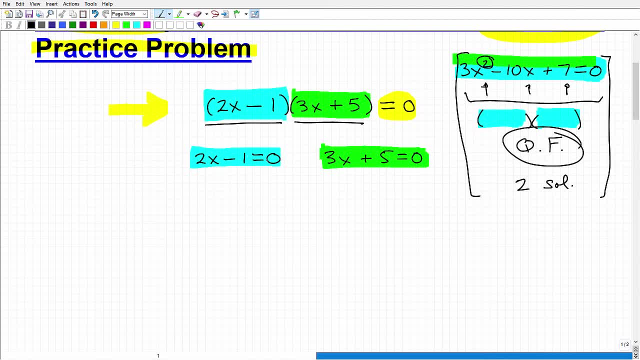 Okay, So hopefully you were able to solve these two little simpler equations, So this one, I'm going to go ahead and add one to both sides. I get: 2x is equal to 1.. I'm going to divide everything by 2.. 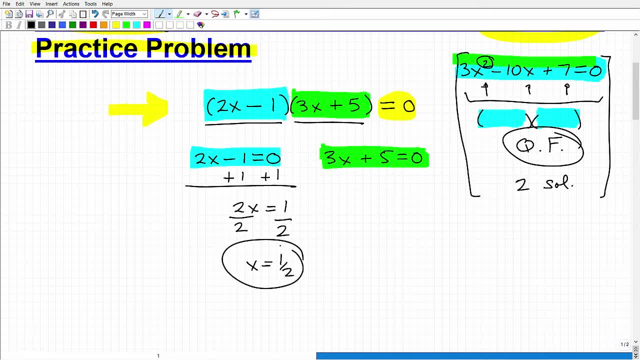 So x is equal to 1 half. That's one solution for this quadratic equation. Let's go ahead and solve for this one. Subtract 5 from both sides of the equation I get 3x is equal to negative 5.. I'm going to divide both sides by 3.. 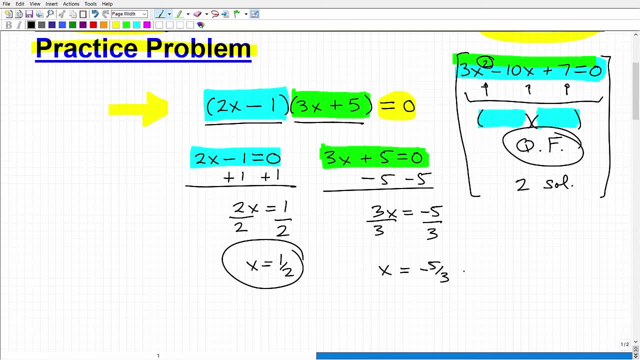 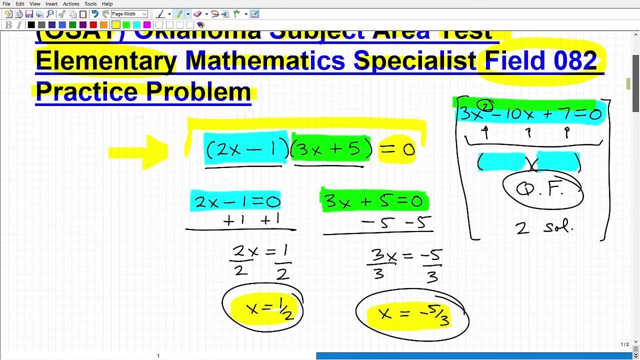 So I get: x is equal to negative 5 thirds. Okay, So these two right here are my solution To this quadratic equation that has been factored for me. Okay, All right. So again, in mathematics, often what looks easy or what can be easy is totally dependent upon your understanding of the subject. 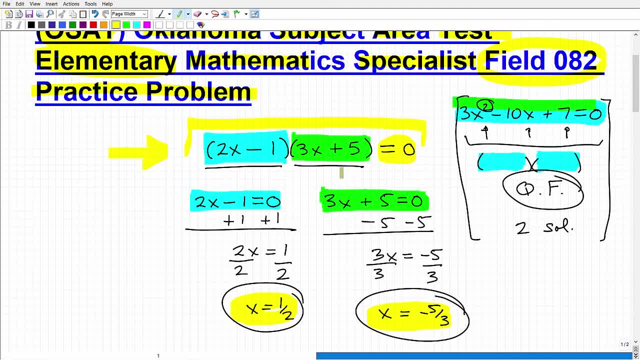 Right. So hopefully you didn't multiply this together and you were doing, let's say, you use the quadratic formula, but you multiply this together, and you actually did that and you solved it. That's pretty awesome. I congratulate you on that. However, that was, you know, kind of going the long route, where this is the most direct route. 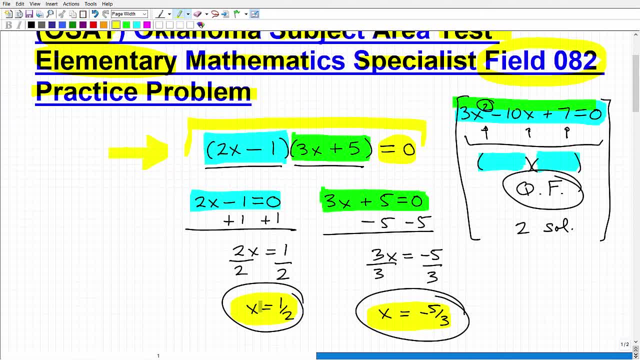 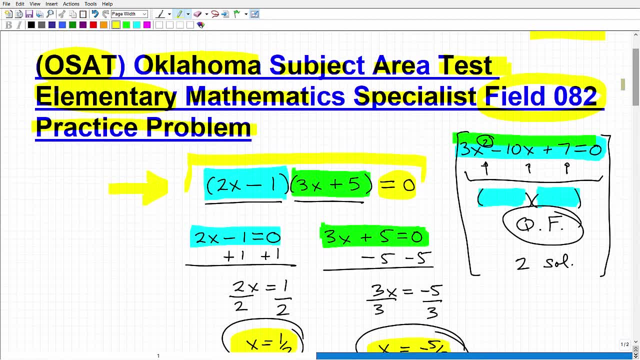 But this is just one example of one subtopic of algebra, of solving equations. There's many, many more other topics that you're going to have to know. for the level of math It's going to be on the OSAT elementary math specialist. 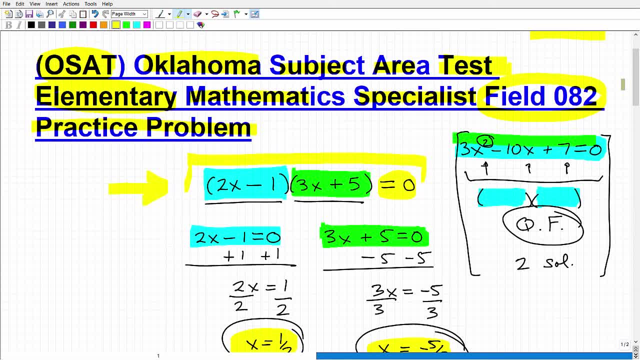 Okay, Again, don't let that word elementary fool you. in terms, Yes, Are you going to be teaching this to third graders? Yes, No, Okay, But are you going to need to know this for your test? Yes, Okay. 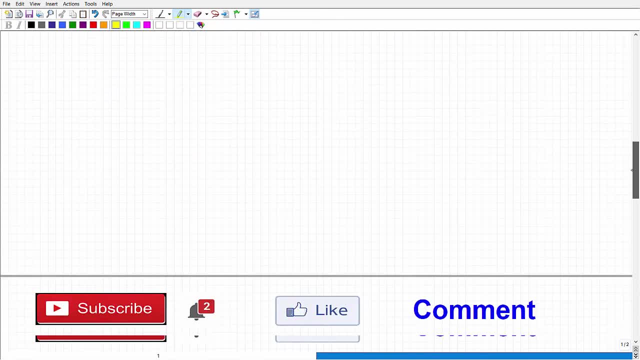 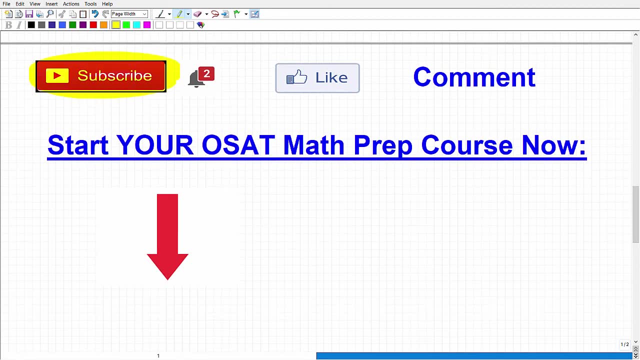 All right. So let's go ahead and wrap this video up. So if you're still with me up to this point, I certainly appreciate it. I've been on YouTube for many, many years, have hundreds and hundreds of videos I post all the time. 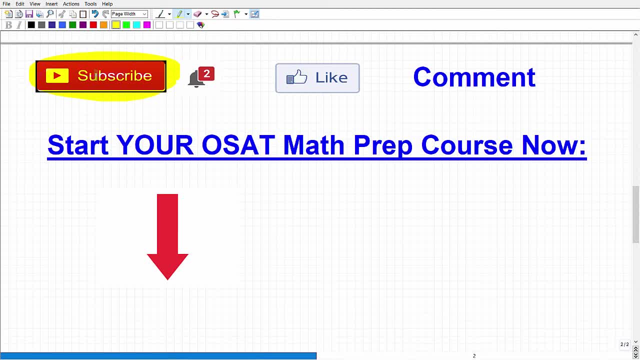 So if you like my videos, like my content, please consider subscribing. I actually have hundreds again on my channel that can help you prepare for this particular OSAT exam. If you enjoyed the video, definitely. I appreciate a thumbs up and leave me some feedback. 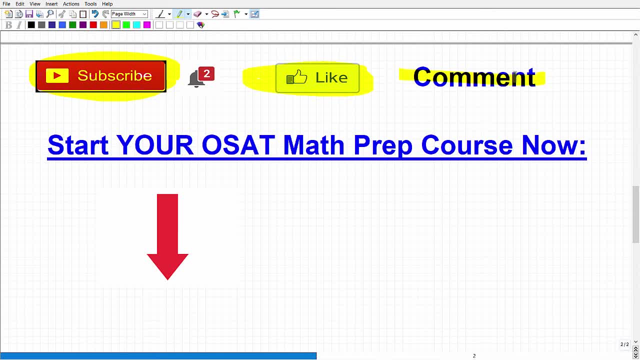 Are you just starting to teach? Are you kind of making a career switch? You know, for example, I started off in high school math and I thought, hey, maybe middle school math would be different or easier. I went to middle school and it was actually more challenging.